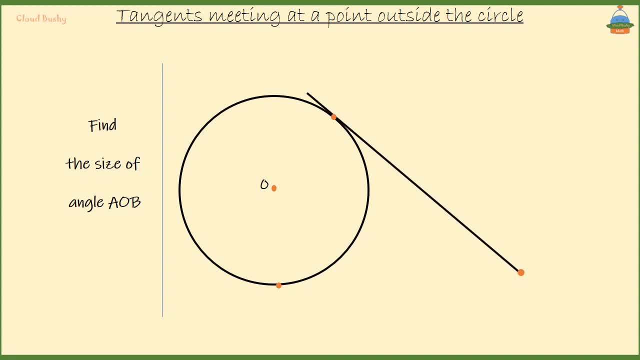 All right. This one pertains to tangents meeting at a point T outside a circle. Let's call these points on the circle A and B. Now, if we draw two radii from the point O at the center of the circle to points A and B, we know that the angle OBT is 90 degrees. So is the angle OAT. 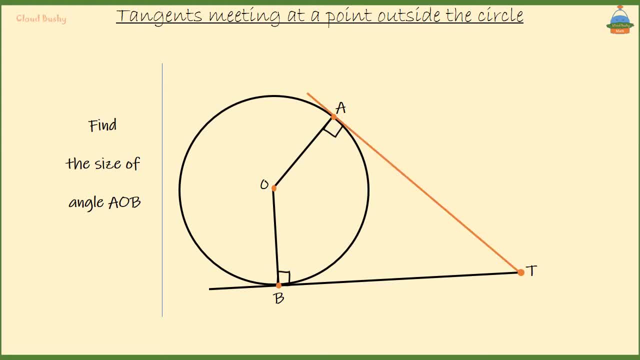 This is because the angle between a tangent and a radius is always a right angle. Now, AOBT is a quadrilateral. It's an angle between a tangent and a radius. Internal angles should add up to 360 degrees. Now, since 90 plus 90 is 180 degrees, these two angles, ATB and AOB, must add up to 180 degrees. 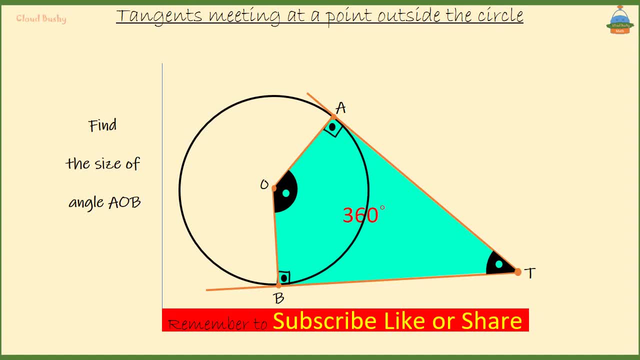 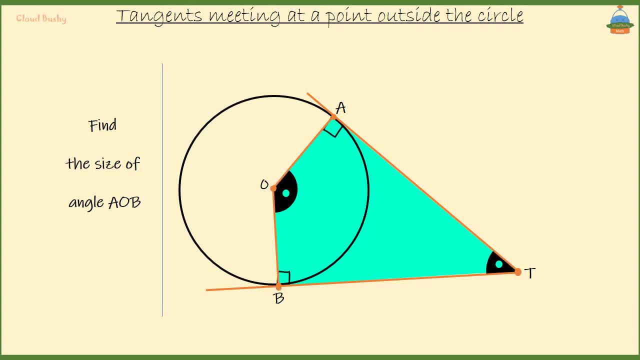 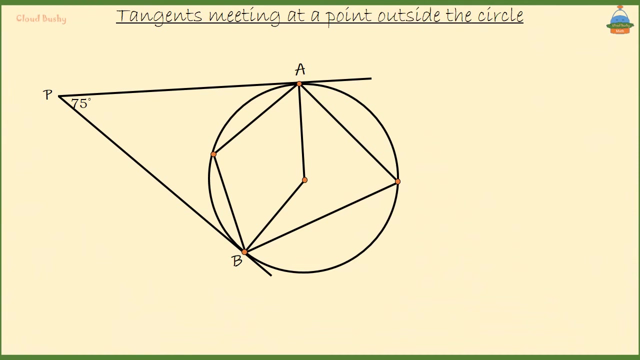 bt. so if angle a, t, b is 70 degrees, it means angle a or b is equal to 180 minus 70 degrees. that gives us 130 degrees. now let's take this further. we have here a circle with two tangents, a, p and b, p. meeting at point p, angle a, p, b is given as 75 degrees. 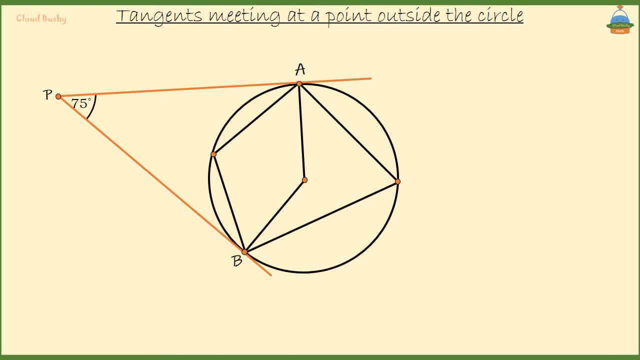 two more points are marked on the circle: point q and point m. 4 is the center of the circle in this diagram. we want to find the size of angle a, t, b and b- t. so if angle a, t b is equal to 180 minus 70 degrees, 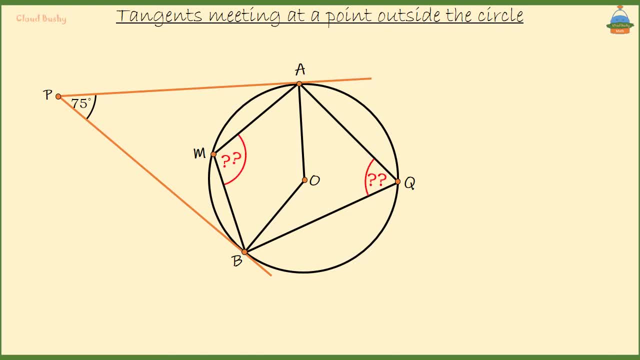 we need to know the size of angle a or b first. now we know that a p b plus a or b should be 180 degrees, because we are sure a, o and o b are radii. we know that the angle between a tangent and a radius. 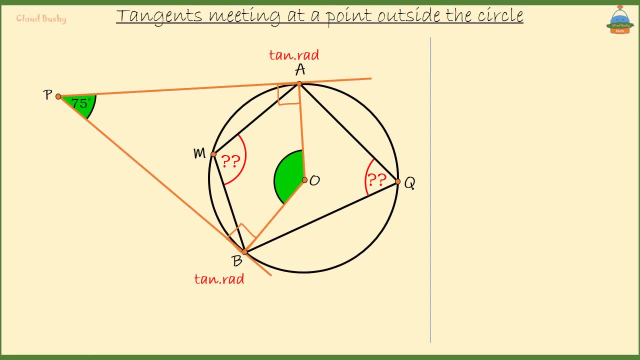 is equal to 180 degrees is always a right angle. so we have 90 degrees plus 90 degrees. now, since 90 plus 90 is 180 degrees, we are only short of 180 degrees if we are to have a total of 360 degrees in this quadrilateral. now, 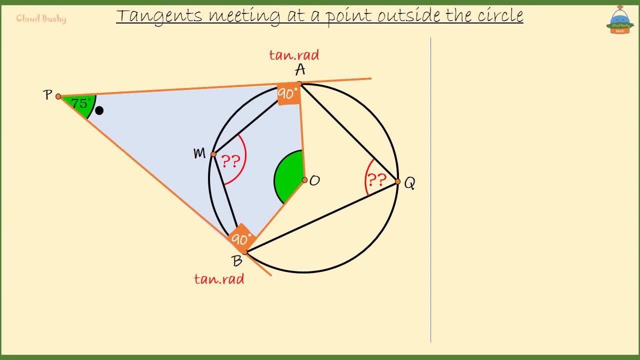